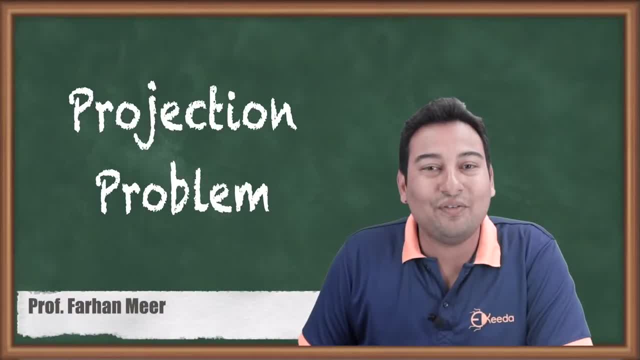 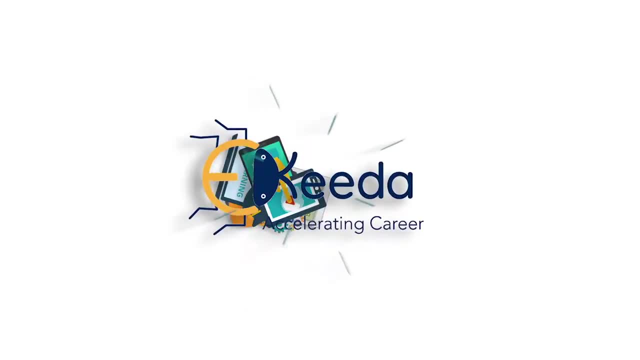 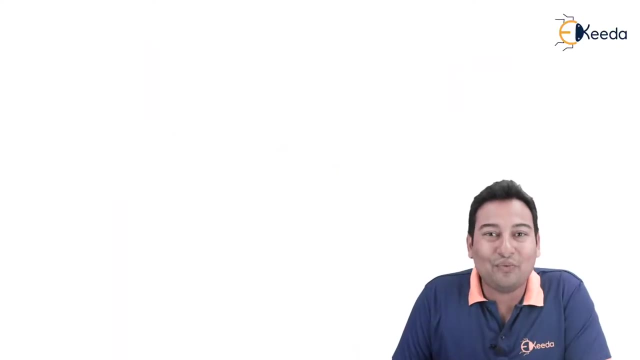 Hello, friends. in this video we'll be discussing vector spaces, in which we'll see what exactly projection is, and we'll see one problem on it. Welcome back, friends. in this video we'll discuss what exactly projection is, because that is very important. that will be required in gram smith method. that is our next time. First of all, 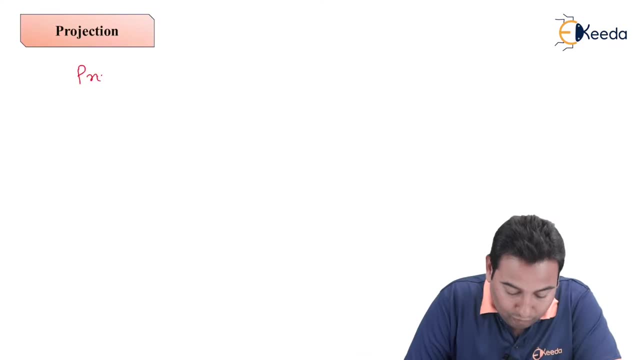 see the formula: projection of u on v. It is written as: projection of u on v is equal to u dot v divided by norm of v square dot v. This is the formula of projection of u on v, and the next formula is projection of u on v. 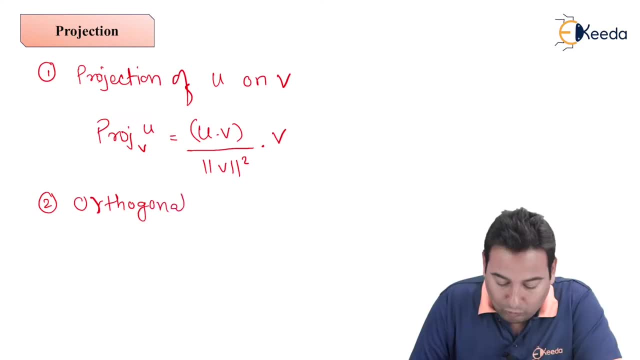 The next formula is orthogonal: projection of u on v is u minus projection of u on v, which is equal to u. minus projection of u on v is u dot v upon its on v. therefore, in denominator norm of v, square dot v. These are the two. 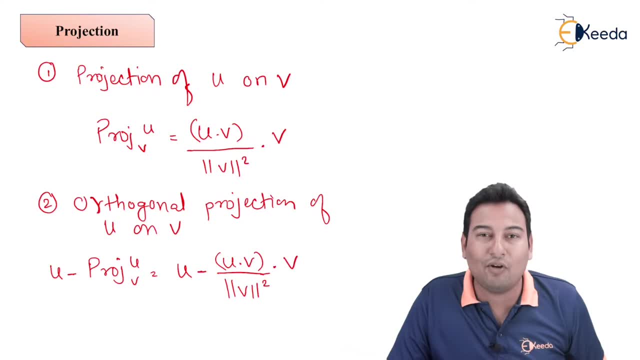 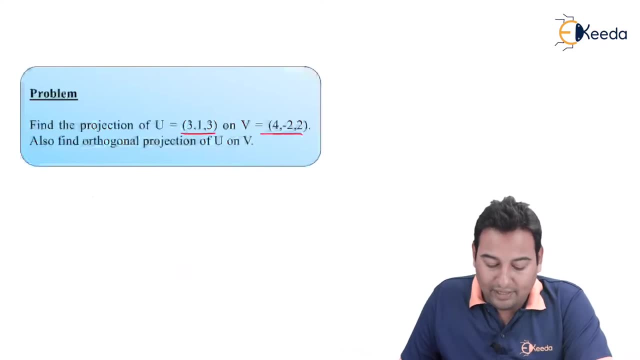 formulas that we'll be using for solving the problem. Let's have a look on the given problem. Here we need to find the projection of u on v. Also, we need to find the orthogonal projection. We discussed the formula here. Now we'll see how to implement this formula. 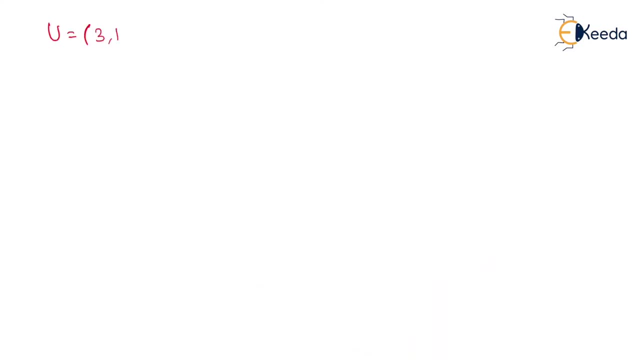 u is equal to 313 and v is equal to 4 minus 2 and 2.. First is we need to find it in the following class. We need to find it in the following class: U dot v times norm of v. square dot v is equal to u dot v. We need to find out: its dot product is 12, 3 x 4, 1 x minus 2 is minus 2,. 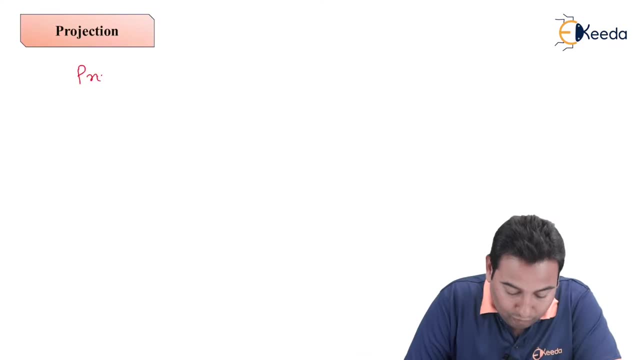 see the formula: projection of u on v. It is written as: projection of u on v is equal to u dot v divided by norm of v square dot v. This is the formula of projection of u on v, and the next formula is projection of u on v. 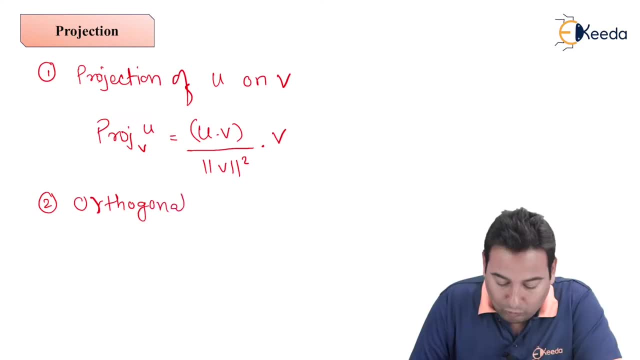 The next formula is orthogonal: projection of u on v is u minus projection of u on v, which is equal to u. minus projection of u on v is u dot v upon its on v. therefore, in denominator norm of v, square dot v. These are the two. 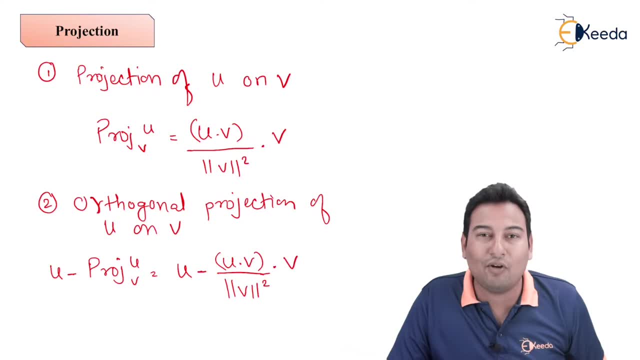 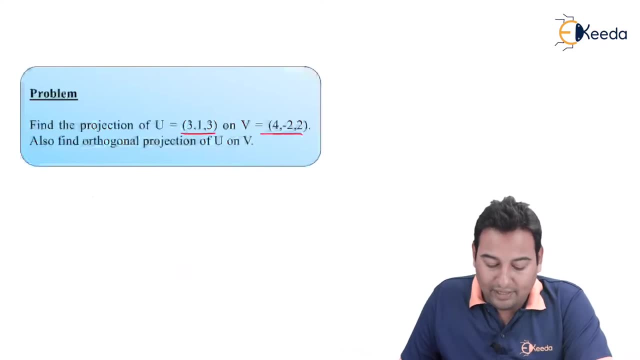 formulas that we'll be using for solving the problem. Let's have a look on the given problem. Here we need to find the projection of u on v. Also, we need to find the orthogonal projection. We discussed the formula here. Now we'll see how to implement this formula. 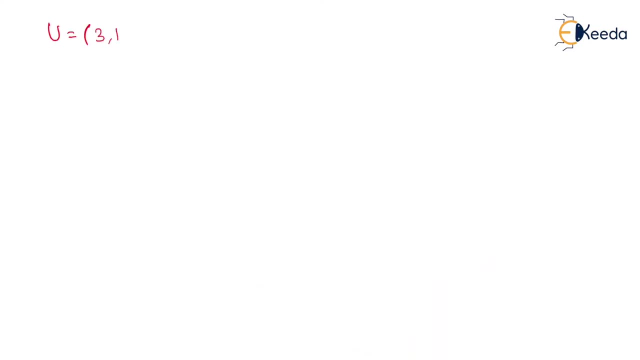 u is equal to 313 and v is equal to 4 minus 2 and 2.. First is we need to find it in the following formula: u is equal to 313 and v is equal to 2 and 1.. Next is we need to find the好啦 f・ v. 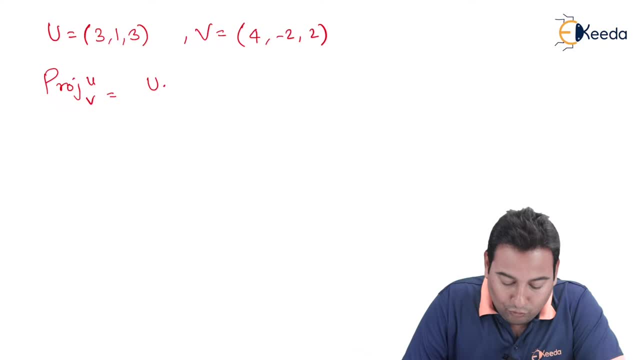 Next, we need to find theבה formula. Know that u is equal to u, dot, v. This is điều supported by norm s Kim Nacortos, whereas V », that is 12, 3 into 41, into minus 2, is minus 23 to Z. 6 upon norm of V, The whole Square. norm means square And that, if you find that u does not give into u, D is not a dropdown. That is a one way as We're going to solve this. You are then going to find the character that's different. one is dot product, that is twelve, three into 4.. One into minus two is minus twoth. two are six upon norm of v. The whole square now means square, wrote, and this is what you'll get. 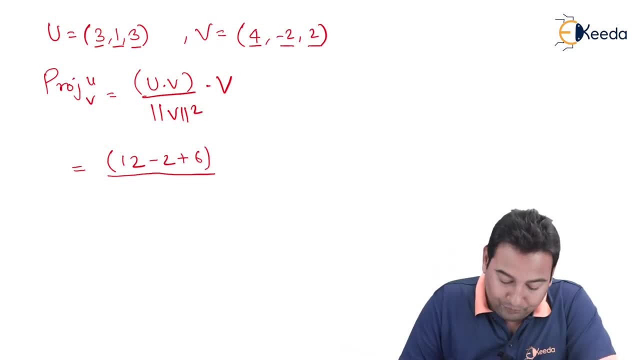 the whole square root and square will be cancelled and we will get 4 square minus 2 square and 2 square, and here it will be v. V is 4 minus 2 and 2, which will be equal to 16 divided by 24, and